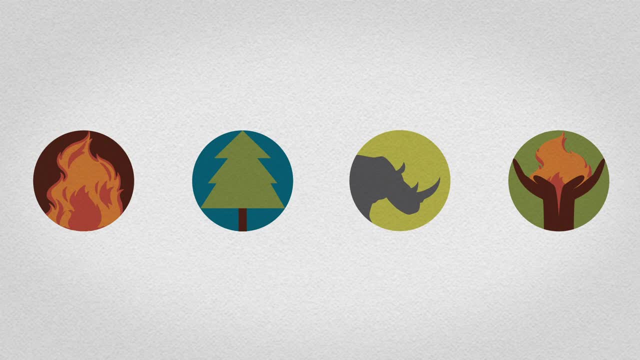 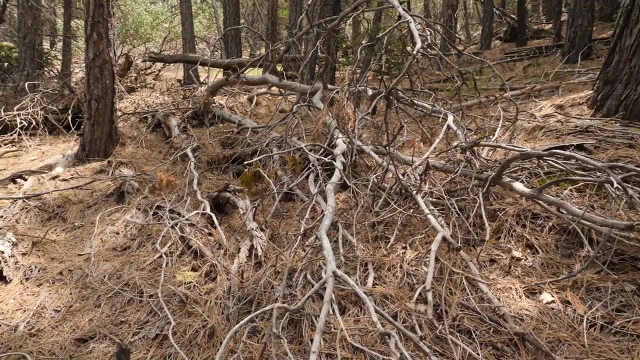 It requires a multifaceted approach For one, we can let natural wildfire fires burn. In some areas, decades of fire suppression have led to a buildup of dry logs and leaves. This can cause out of control blazes- Places like Yellowstone National Park in the United. 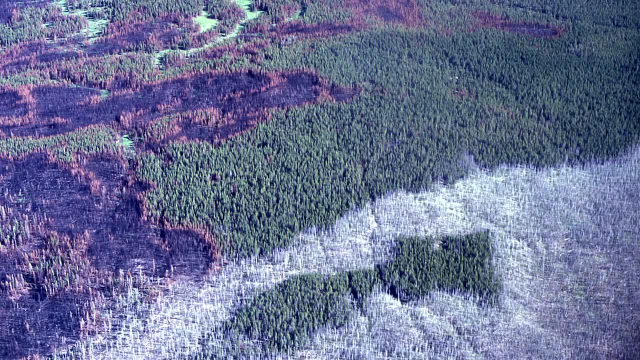 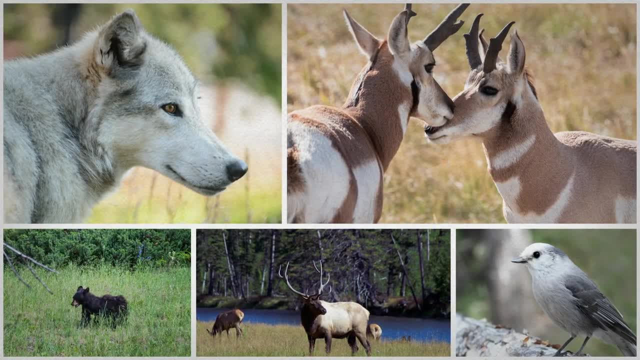 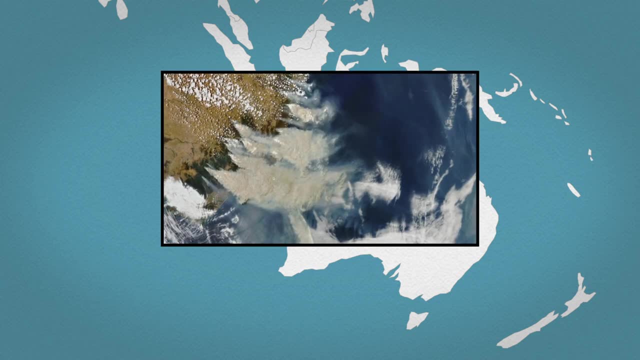 States are allowing small natural fires. These make a patchwork of burned and unburned areas That increases the kinds of plants and animals that can thrive there. When fires do rage, we can protect areas that may not be able to survive During the 2019-2020 Australian fires. 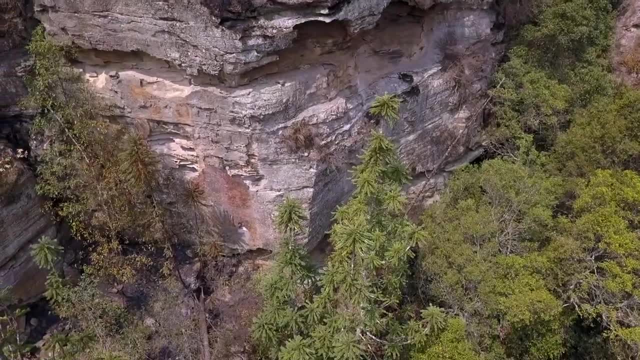 firefighters have been able to stop fires and burn down trees, trees and trees. in the Amazon, Firefighters work to save a grove of prehistoric trees called Willamie Pines. Fewer than 200 of these trees exist in the wild. 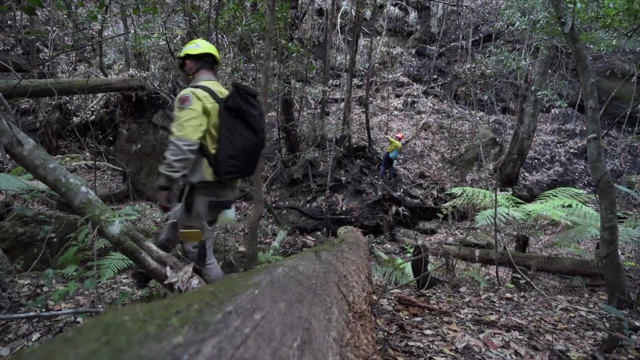 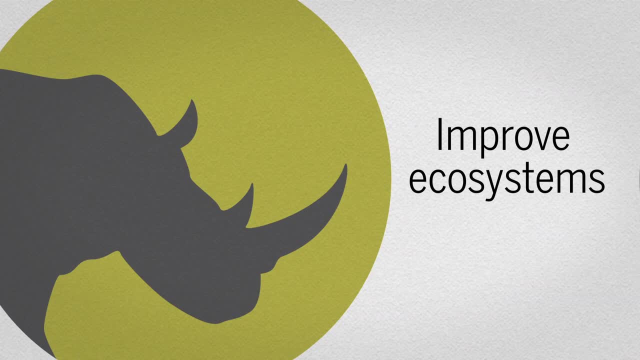 Firefighters set up irrigation to keep the grove wet and surrounded it with fire retardant. They managed to save the trees. We can also try to improve the health of each ecosystem. One way is to reintroduce and protect animals that are important to their habitats. 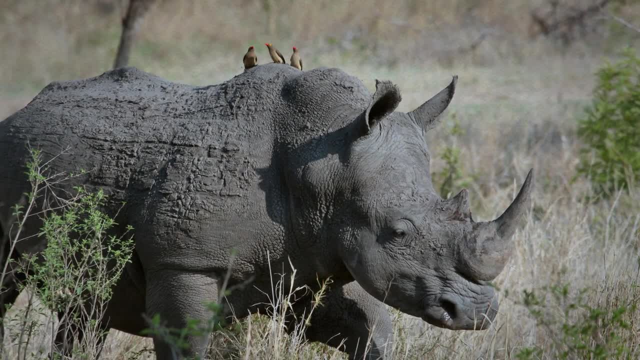 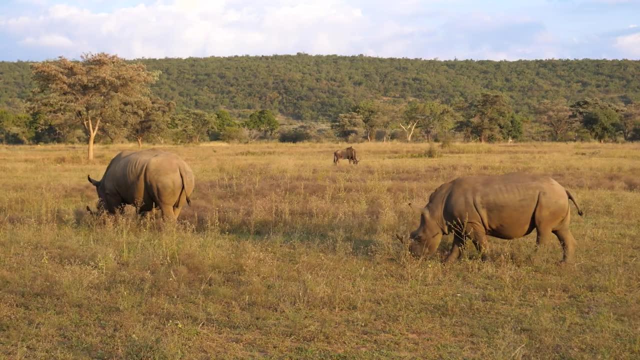 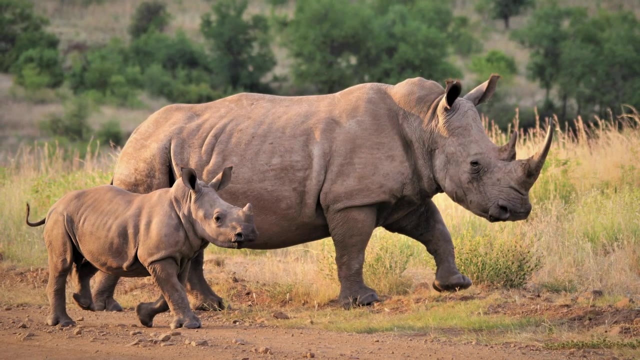 In South Africa, researchers found that fires were 50 times smaller when rhinos grazed the land. Rhinos kept plants from growing out of control. Their paths created firebreaks or gaps in vegetation. Large grazers like the white rhino can rebalance ecosystems and reset their fire regimes. 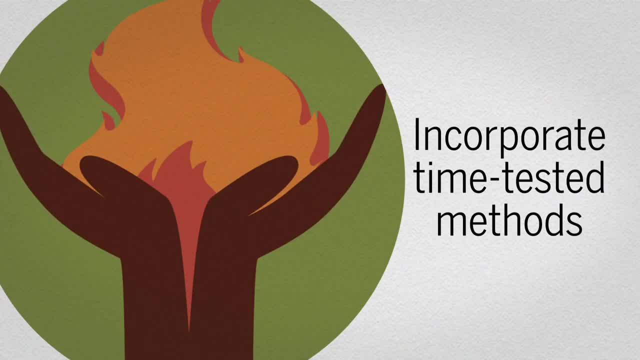 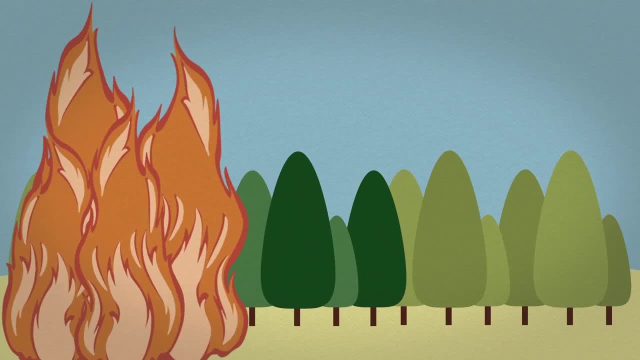 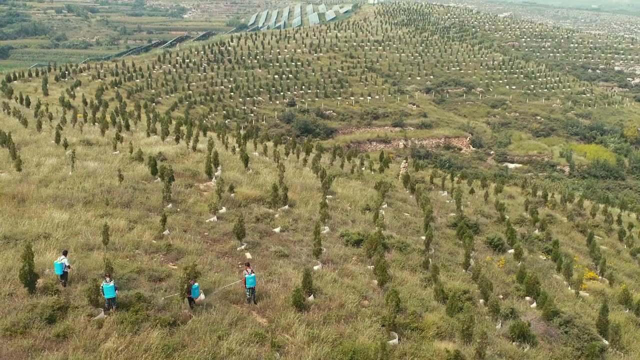 Finally, we can lean on ages-old fire approaches. In China, people have planted green firebreaks to manage wildfires for over a thousand years. These sections don't burn as easily as their surroundings. Recently, the Chinese government planted more than 364,000 kilometers of green firebreaks. 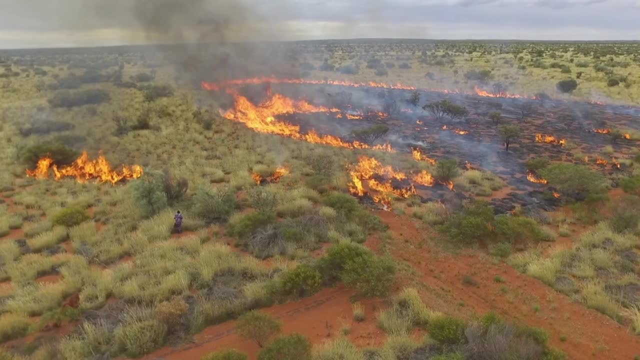 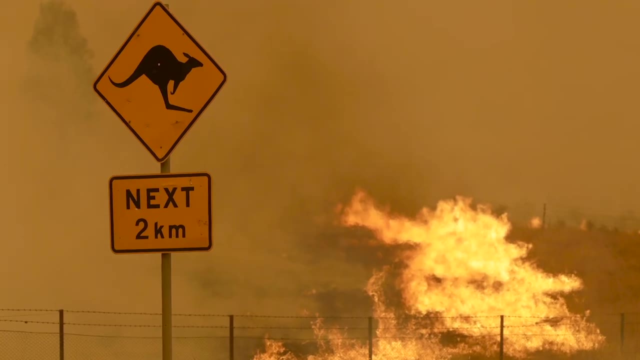 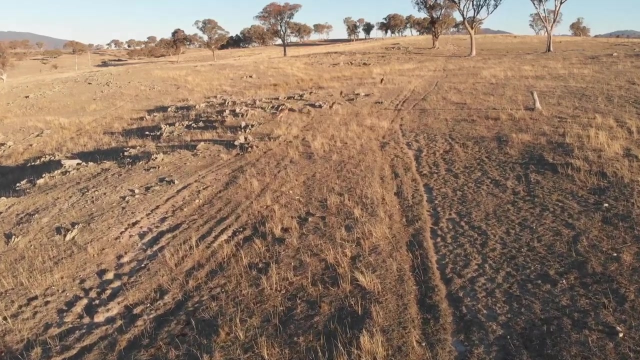 Indigenous Australians have lit fires in the bush for 50,000 years to hunt clear paths and invigorate the land. Areas without these, fires have larger and more dangerous blazes that are triggered by lightning. Using Indigenous strategies for the land can help manage fires in a sustainable way. 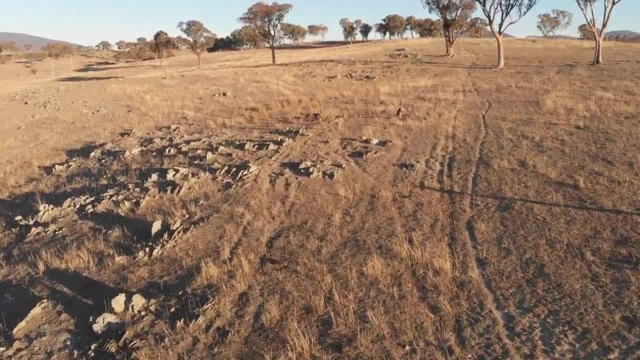 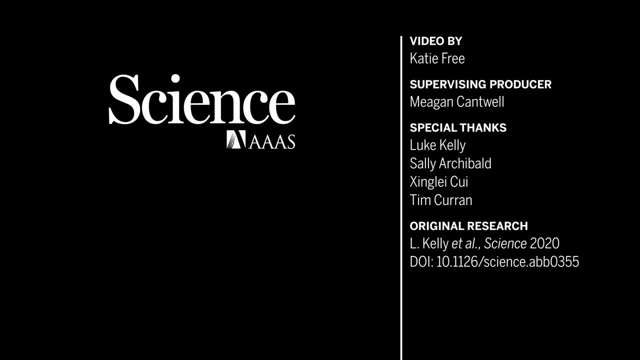 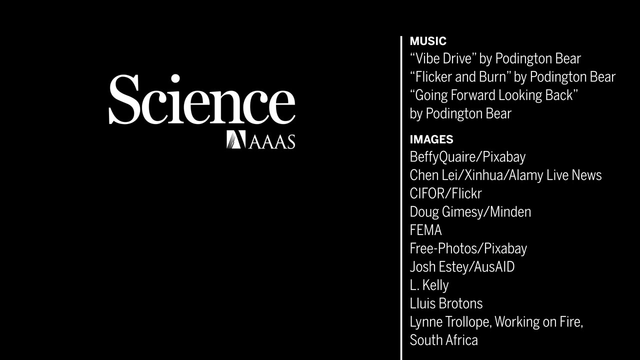 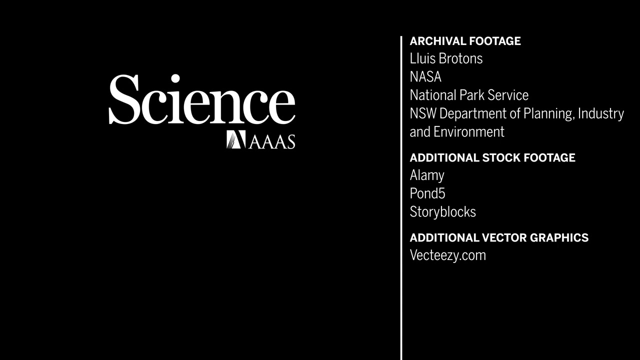 Challenges are ahead, but an integrated approach to fire may help us and the planet. For more UN videos, visit wwwunorg.